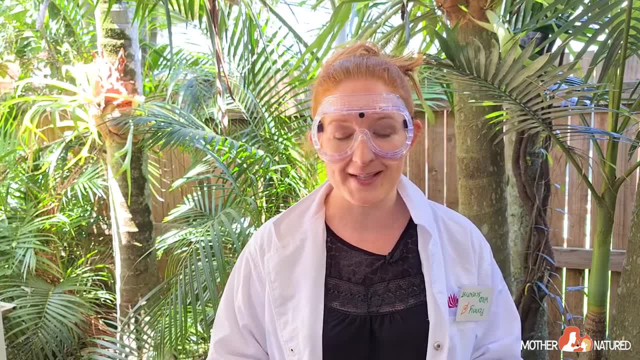 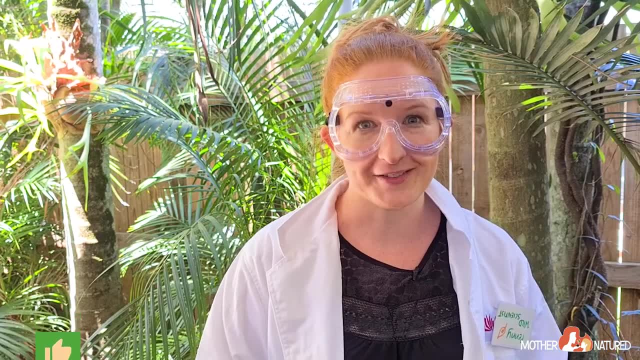 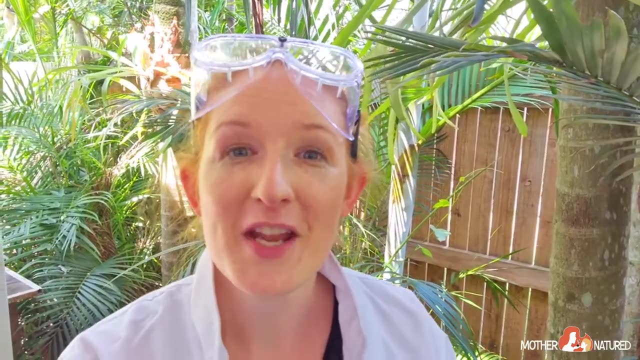 But it turns out an animal kept stealing our grapes, so he became the experiment. Don't worry, no animals were harmed when we made this video, And if you want to find out who became our experiment, you'll have to watch until the end. For this experiment, you need a few small leaves. 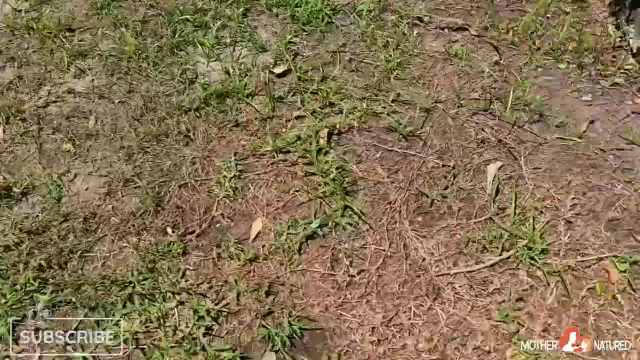 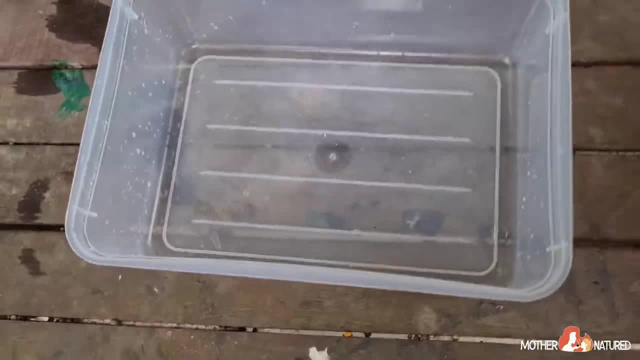 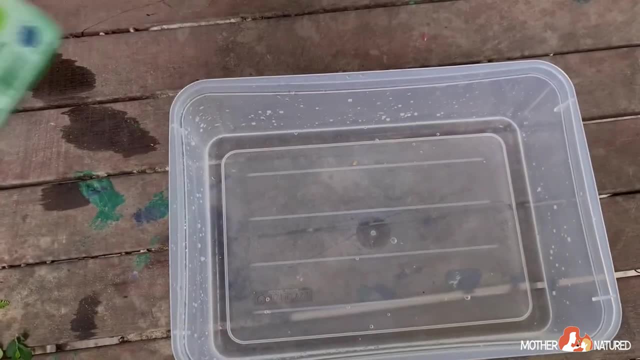 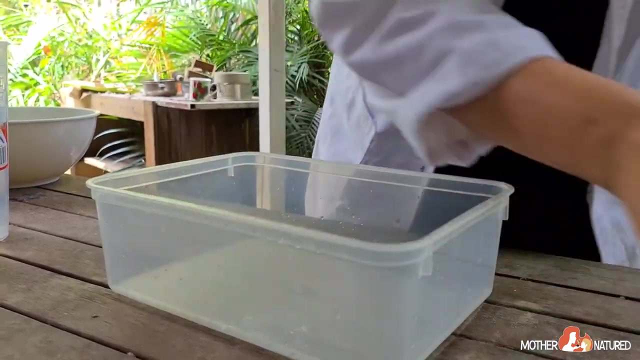 Try a few different types. Let's go and grab some. Here's what you need: A large container filled with water, liquid dish soap, a few small flat leaves and a little stick. Put a big dollop of fish soap on the end of a stick and then smear it. 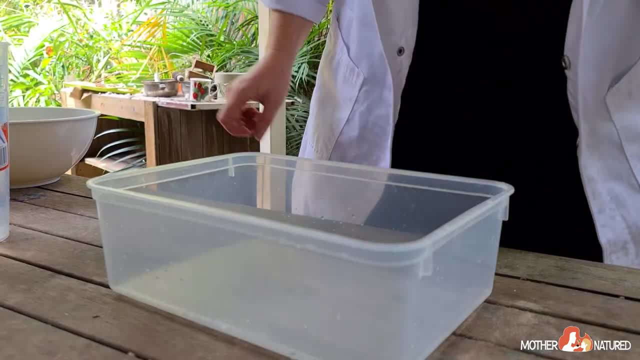 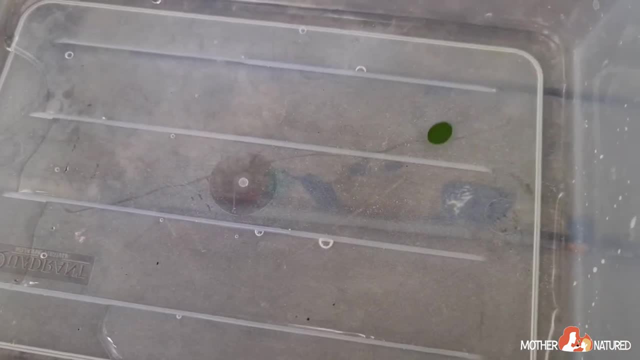 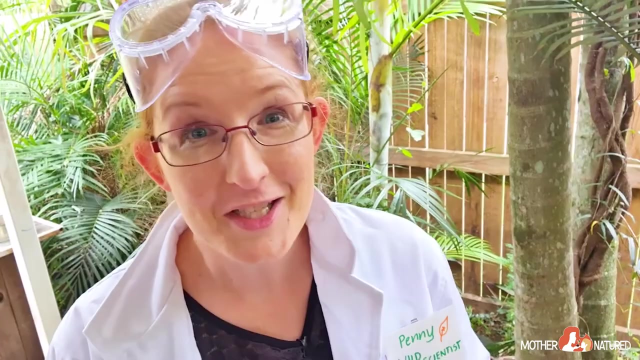 on to the end of one of the leaf tips. Now gently place the leaf in the water. What's happening? The soap contains sulfactants which lower the water's surface tension. The soap has a force of attraction between the leaf and the water which makes it fail. Placement of the soap. 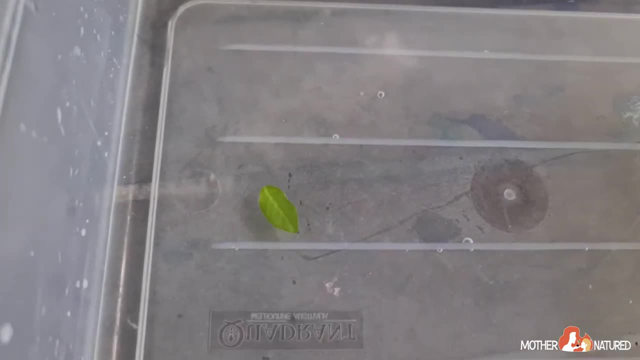 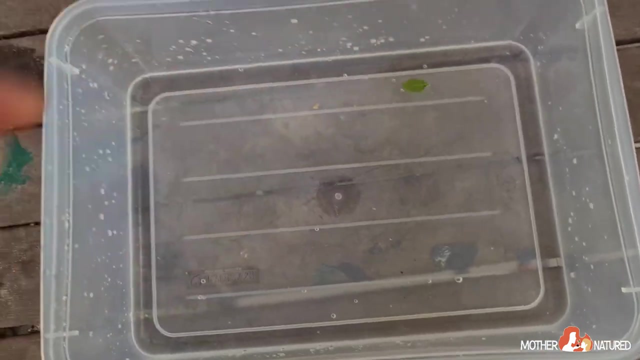 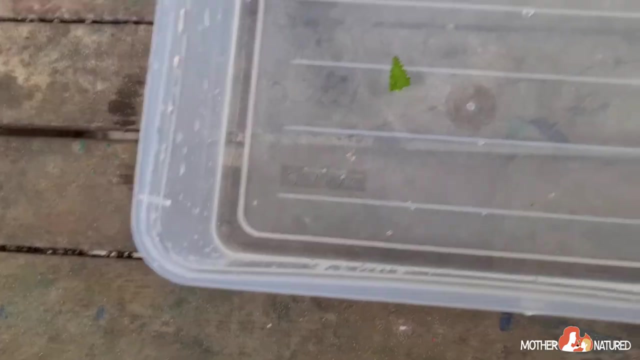 in the small notch at the back of the boat means that the only way for the soap to disperse is by moving out the back, causing the leaf boat to move across the water. The boat moves by being pulled forward by water molecules rather than being pushed by soap molecules Since the surface. 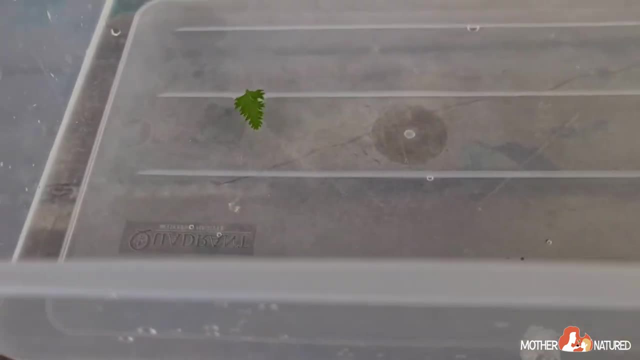 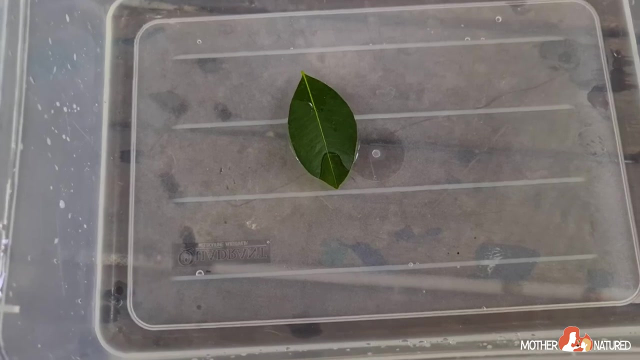 tension is greater at the front of the boat than at the rear, it pulls the boat forward. Once the soap has spread out across the surface of the water, the boat will stop moving forwards. The leaf that worked best for us and went super fast was like the little leaf with tiny little. 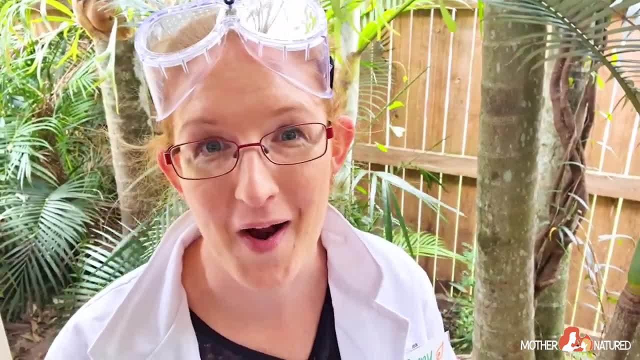 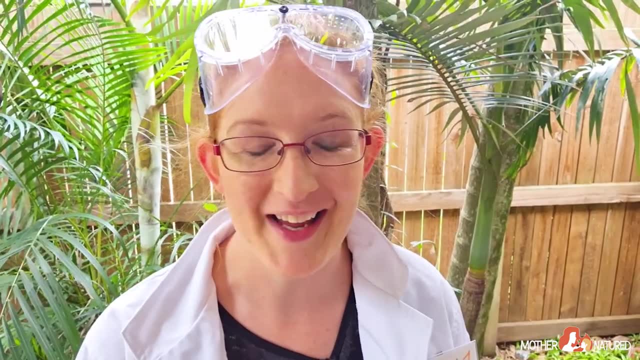 hairs on it, It seemed to really zoom around for quite a while, whereas the big leaf hardly moved at all. Why don't you and your grown-up give this experiment a try? It's super easy and it's really fun trying it with different leaves. 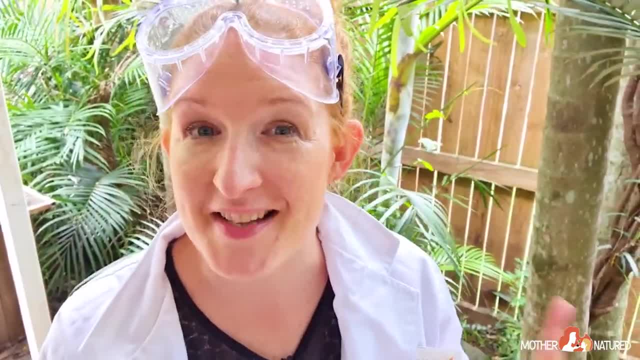 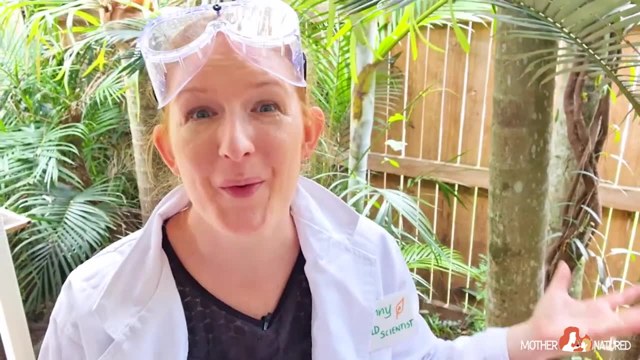 So now we're going to make a material that's both a solid and a liquid, and it just depends on how you play with it as to which it becomes. It's so cool. It's called goop, but it's also sometimes called obleck as well. Have. 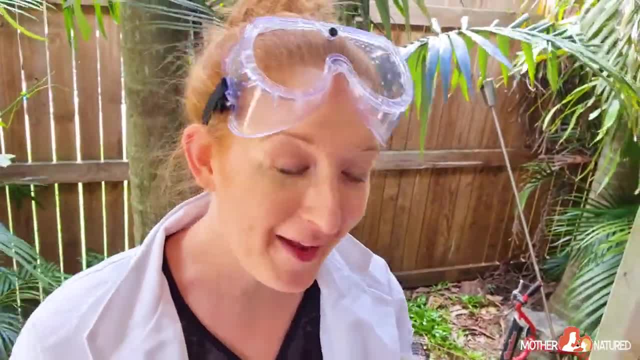 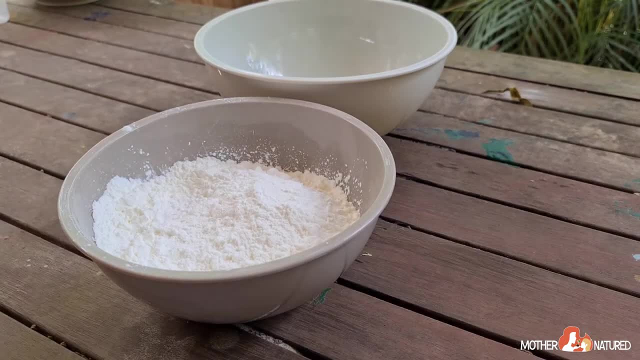 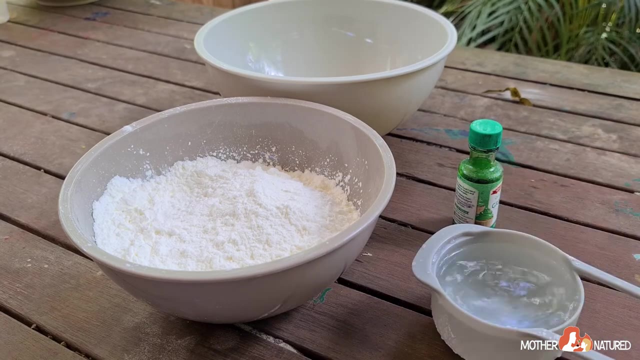 you played with it before And today I had some help, because my kids love messy play too. Here's what you need to make: goop: One and a half cups of corn flour, one cup of water, a bowl, and you might also like to add some food colouring too. Put the cornstarch into the bowl. Now add a. 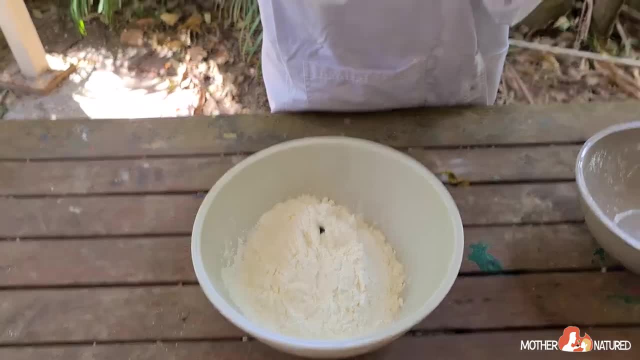 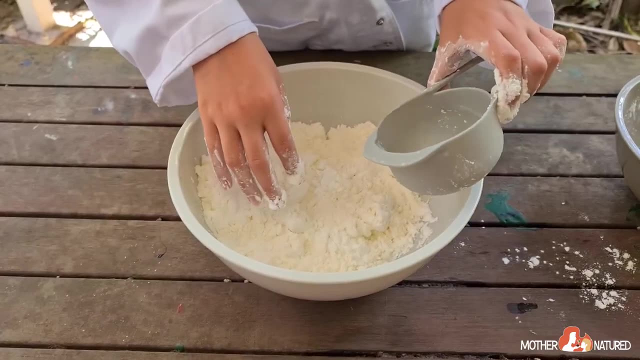 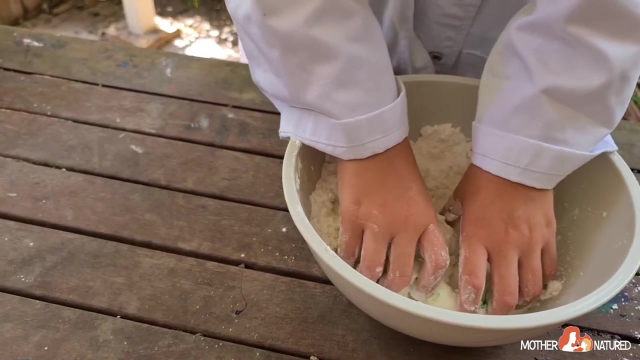 drop or two of food colouring. We're going with green. Add in water, slowly mixing the cornstarch and water with your fingers until all the powder is wet. Keep adding water until the ooze feels a little like a liquid when you're mixing it slowly. When the ooze is just right, it won't splash. when 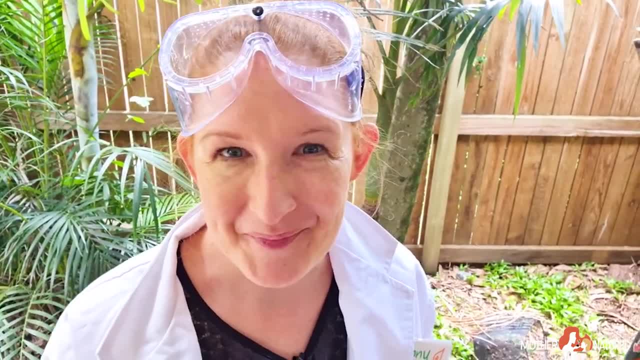 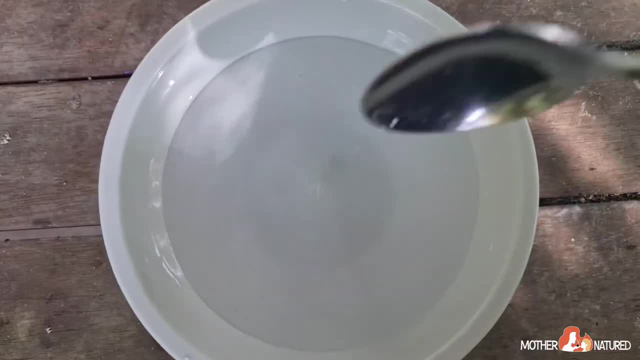 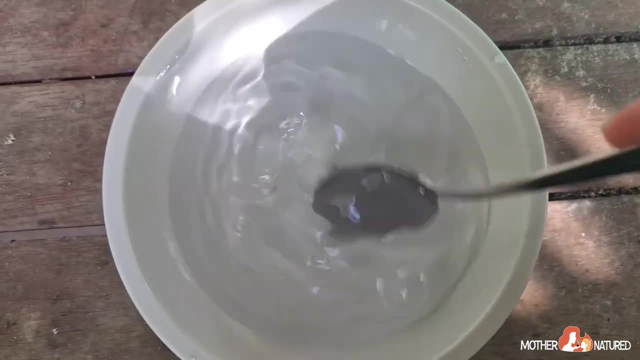 you hit it with a spoon, When the ooze is just right, it won't splash. when you hit it with a spoon, Then you know it's playtime. If you stir a cup of water with your finger, the water moves out of the way easily and it doesn't matter whether you stir it quickly or slowly. Your ooze is made up of tiny 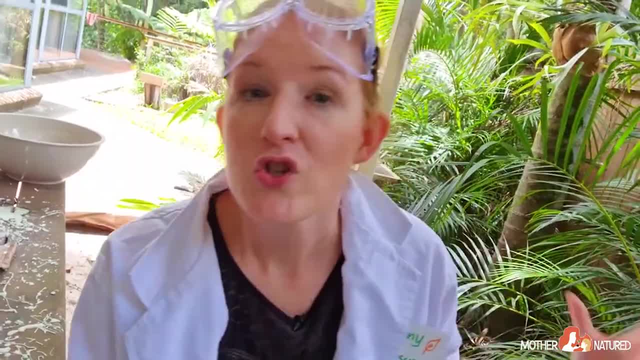 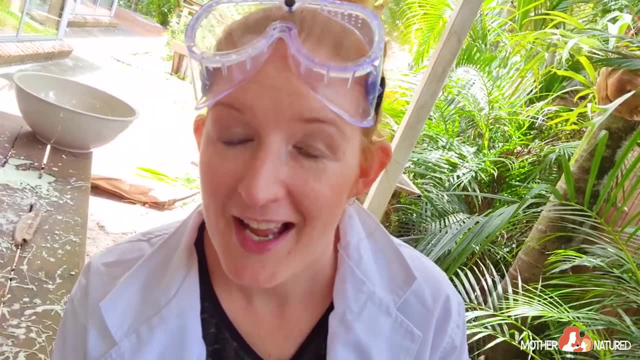 particles of cornstarch suspended in water. So what's going on here? Well, when you put pressure on the mixture, it's incredible. You can add more water if you don't have a mixer. So what's going? it's increasing its viscosity. 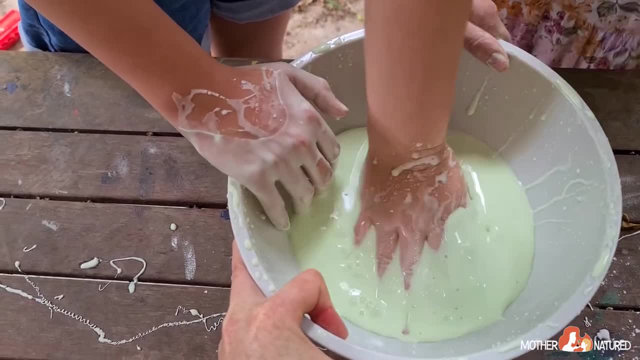 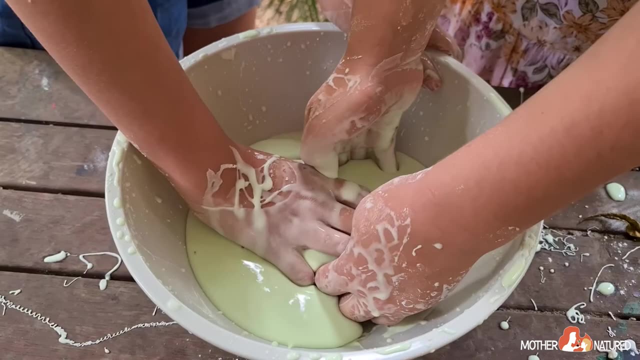 A quick tap on the surface of the goop will make it feel hard because it forces the cornstarch particles together. But dip your hands slowly into the mix and see what happens. Your fingers slide in as easily as though it's water. Moving slowly gives the cornstarch particles. 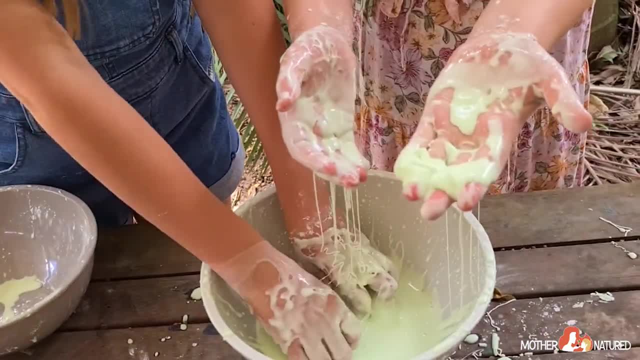 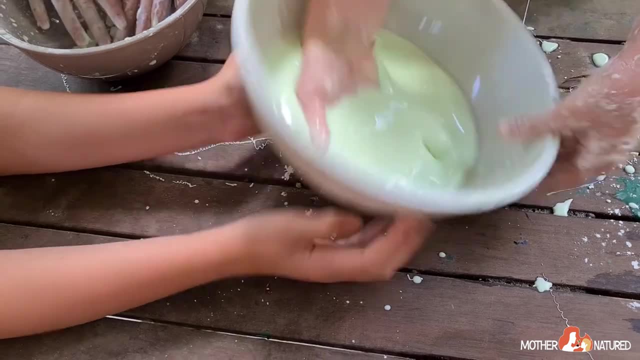 time to move out of the way. Pick up a handful and squeeze it Now. stop squeezing and it will drip through your fingers. Rest your fingers on the surface of the ooze, Let them sink down to the bottom of the bowl. Then try and pull them out as fast as you can. 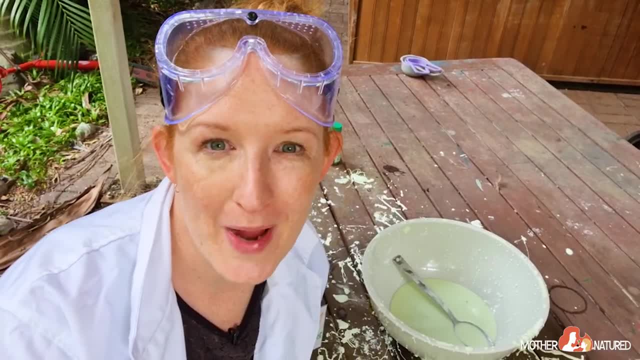 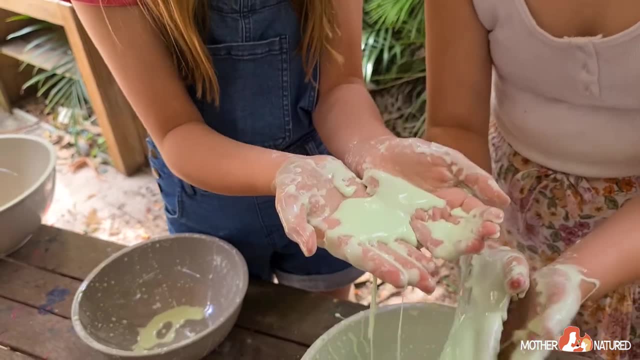 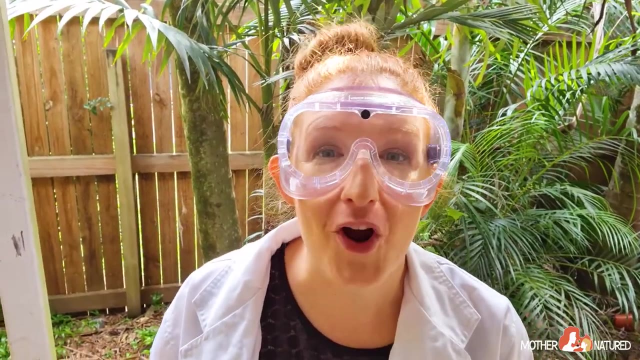 What happens Now. take a blob and roll it around in your hand really fast until it makes a ball. Now stop rolling it and watch as the liquid drips off your hands. You have to try this with your grownup. My daughter wanted to try more experiments. 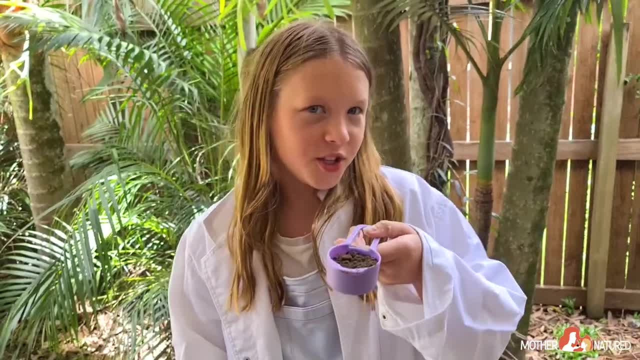 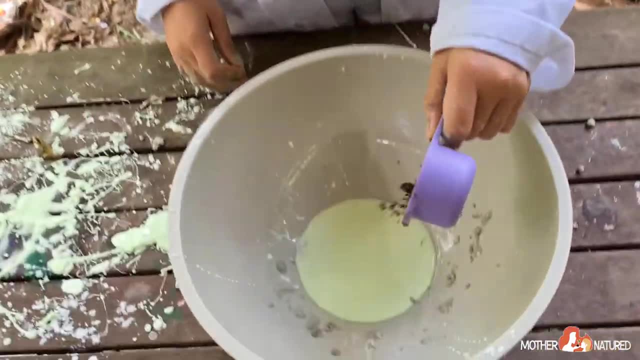 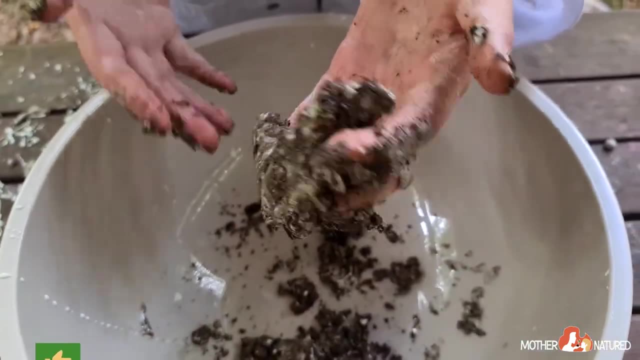 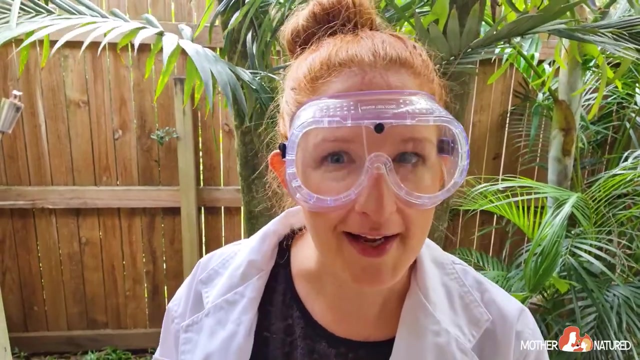 with the goop or oblate mixture. So we're gonna add our goop Dirt into the oblate and mix it around with our dirty hands. It actually feels like clay. it's so cool. You might like to add another substance into your oblate mixture to see what happens too. 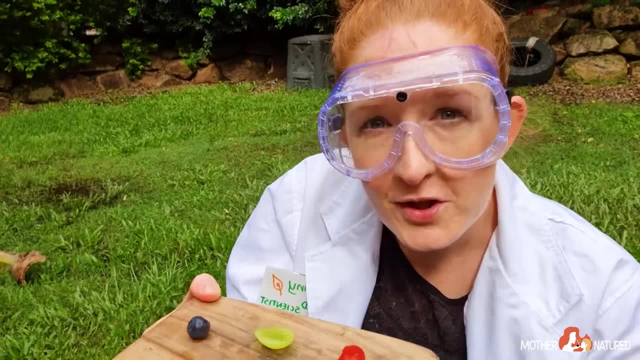 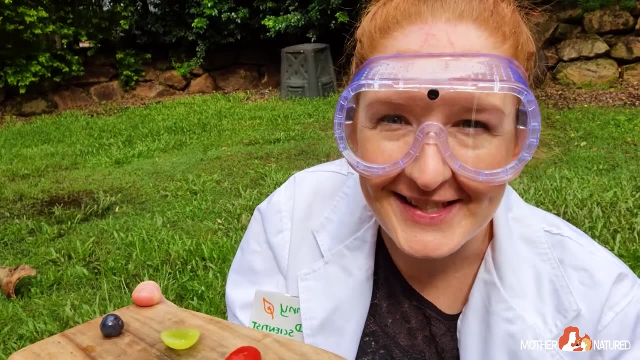 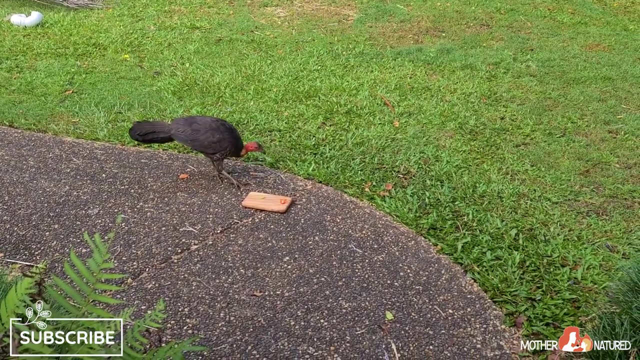 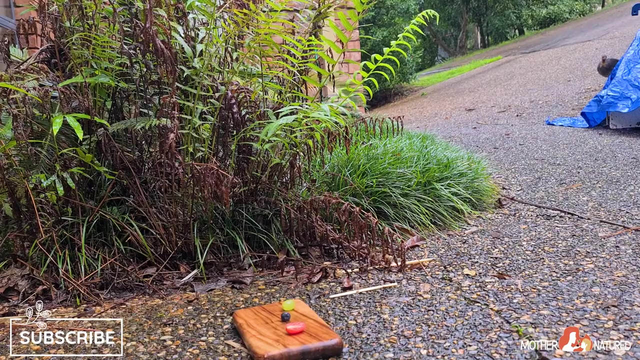 This is Heihei. he became our experiment. Heihei is our favorite plant And we want to know which food Heihei liked best: Tomato grapes or blueberries? I forgot to mention that Heihei is a wild Australian, bush, turkey. 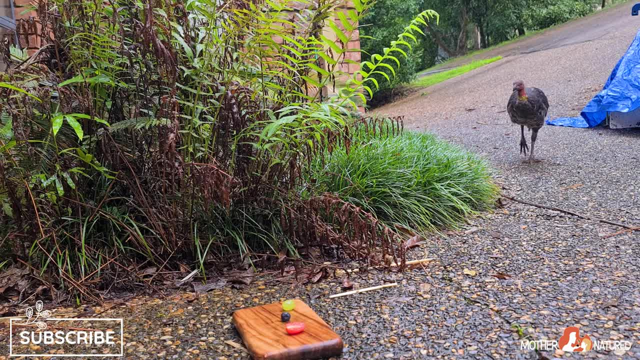 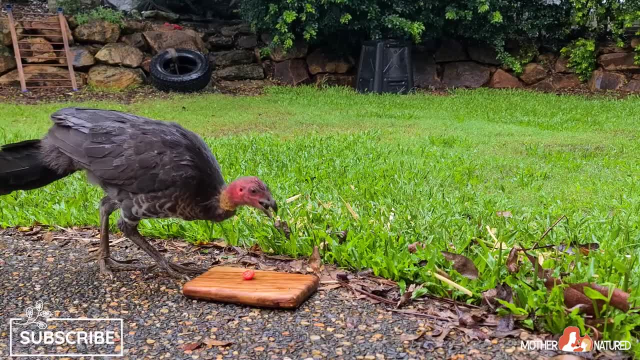 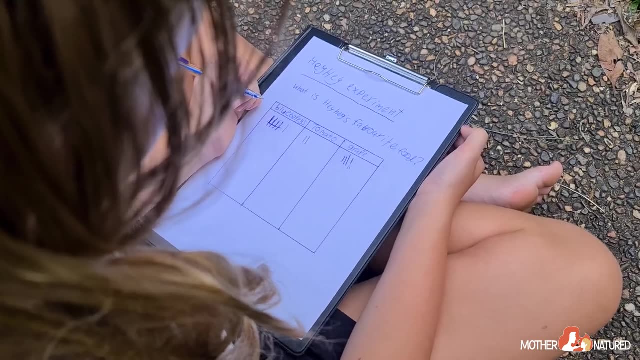 And we live in his territory so he visits often days. we started to wean him off the foods that we were giving him so that he had to find all the yummy, nutritious food on his own. we recorded the findings on a piece of paper and tallied up all. 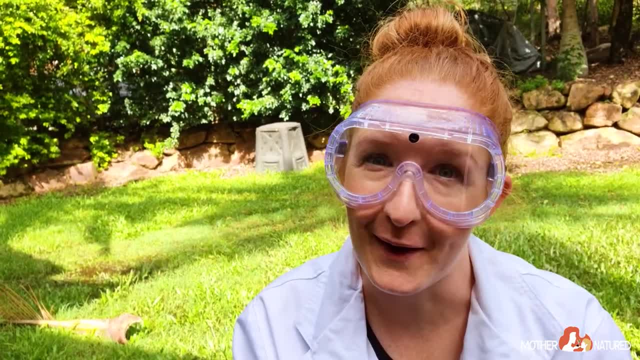 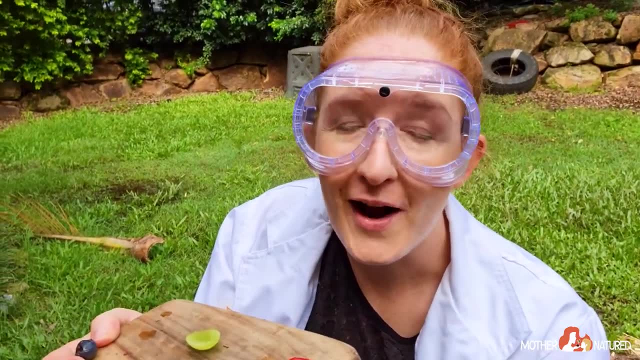 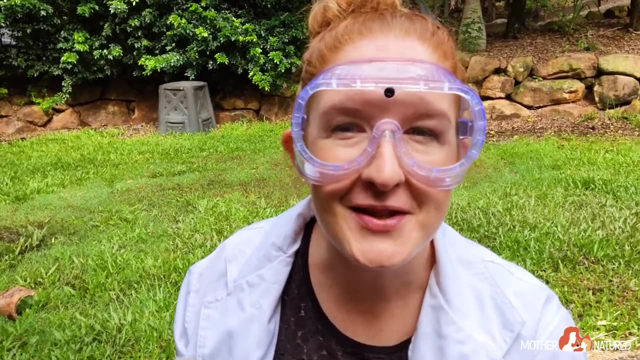 the results. it turns out heihei loved blueberries best and i don't blame him, but he did love all the foods that we laid out for him. you might like to try your own animal experiment. with your grown-up, you could learn more about your family pet or one of the wild animals that visit your garden. 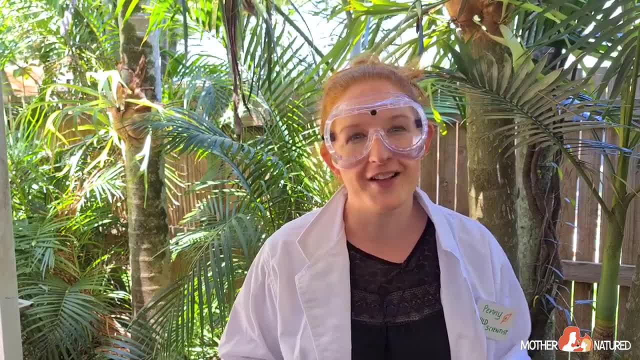 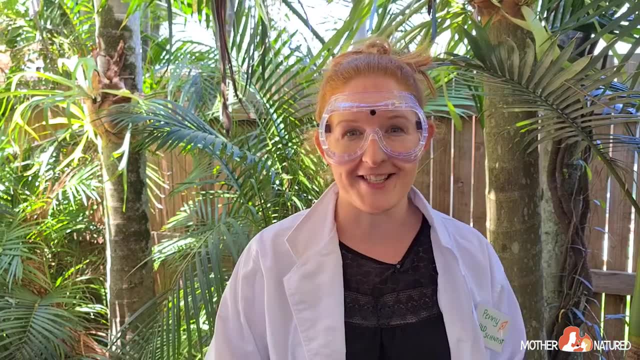 thanks for being here with me today. i hope you enjoyed all the wild nature experiments that we just did. it was a lot of fun. what's some burning questions that you have about nature? why don't you go for a walk in your local area and see if any questions come to mind, and then all you have? 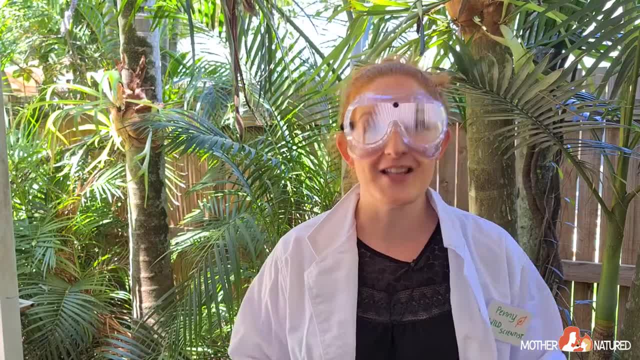 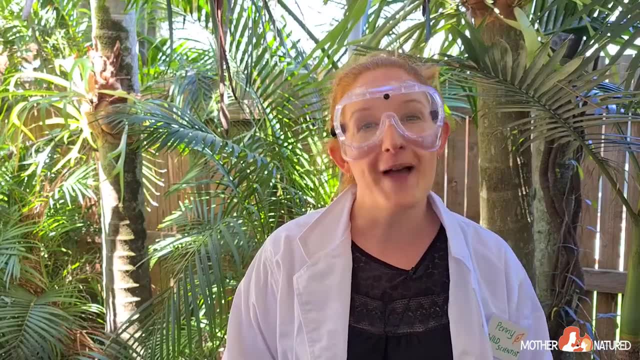 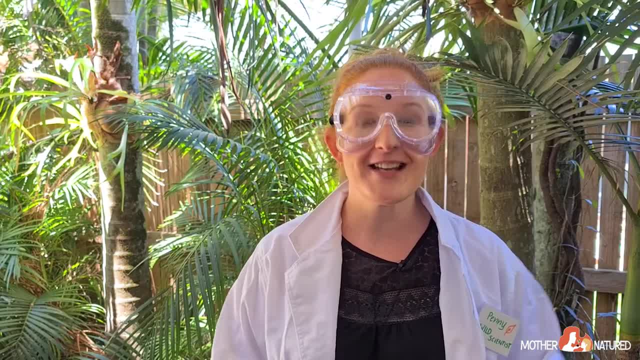 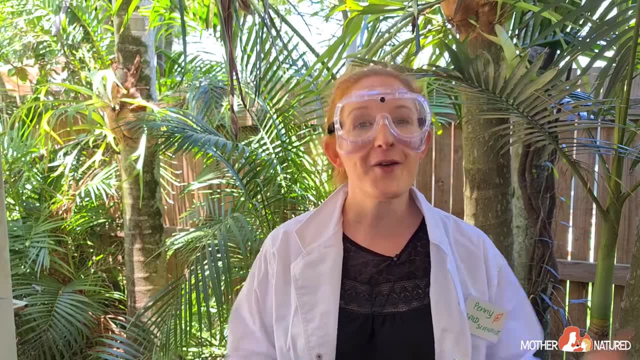 head to mothernaturecom. This is where I support parents and educators with a whole bunch of printables and resources to help get your kids outside. The links are in the caption below, And don't forget to give this video a like.